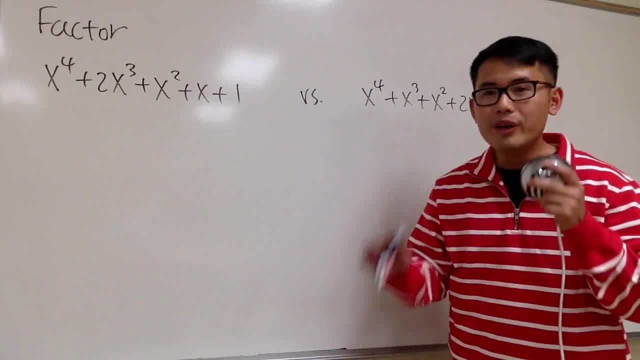 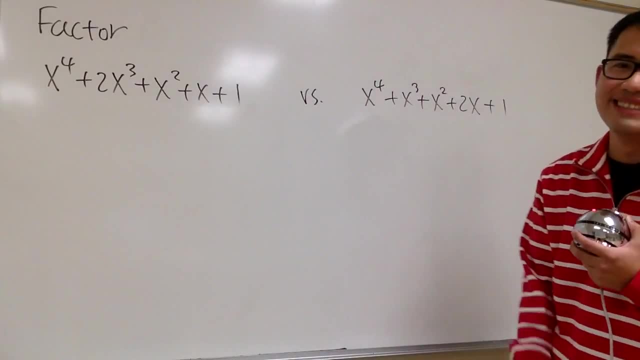 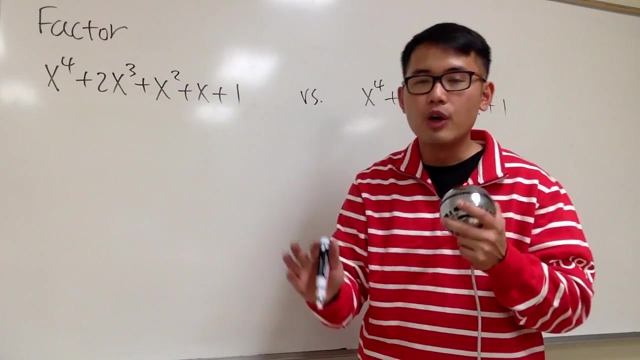 First, not all the five-term polynomials are factorable. We can only do the ones that are well-designed, And second remark is that they will be hard. Anyways, let's focus on this one first. As you can see, we have five terms. As a good habit, we should check to see if we can factor. 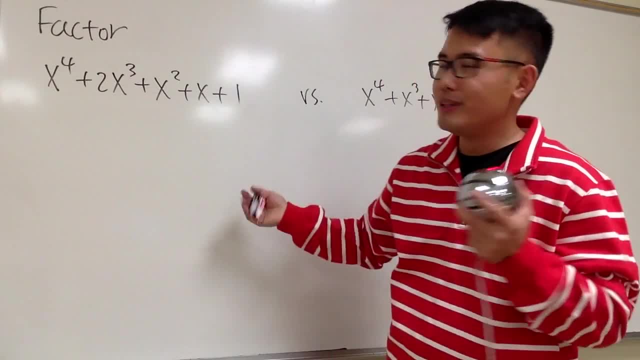 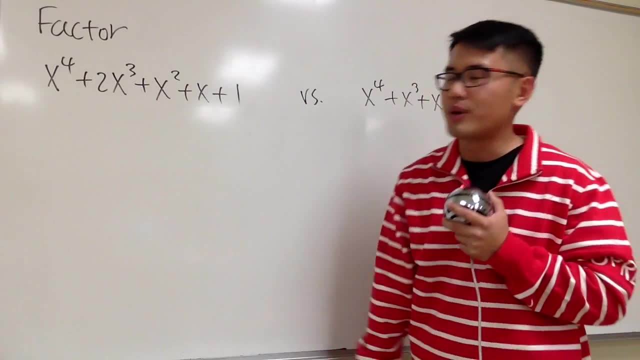 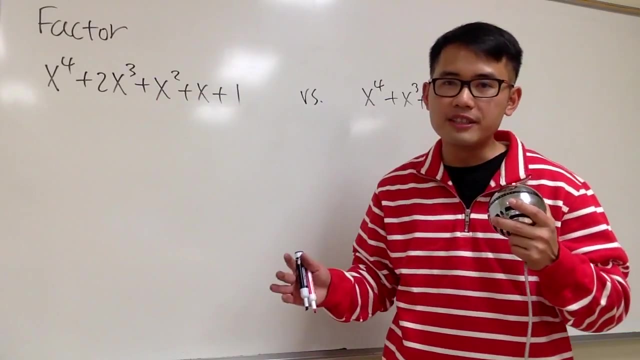 any GCF from all these terms? But no, because first of all, the last one is just a one, and then for the numbers, there's no other number besides one. right. So no GCF, And right here, whenever we're trying to factor things out, that has more than three terms. 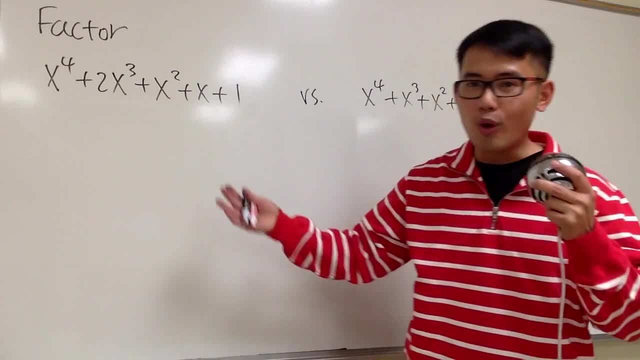 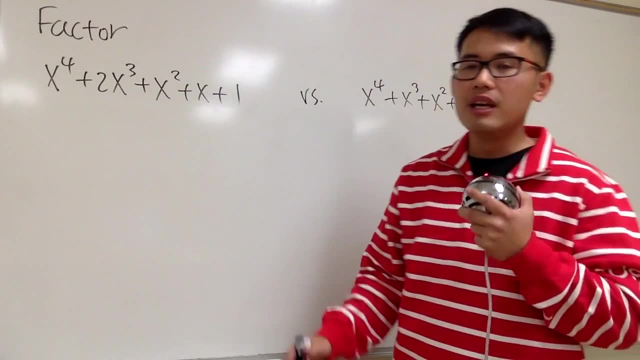 and that means if we have four, five, six or even more, we should do this by grouping This right here. we have five terms and we have a few ways to group them right. Maybe you can group the first two together. 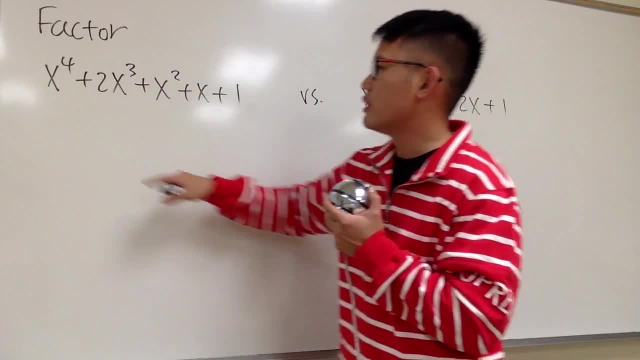 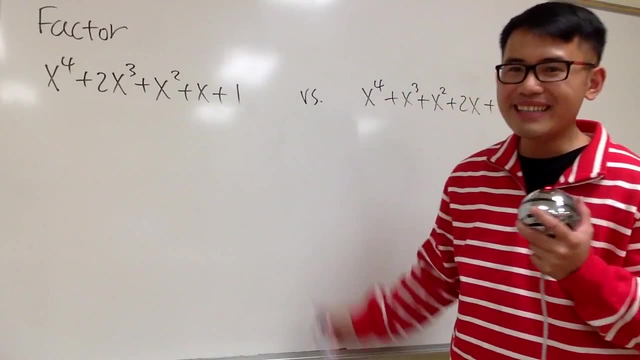 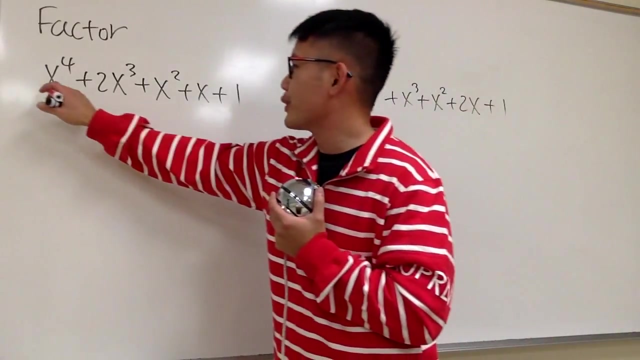 and then the second three like this, or the first three like this, and then the last two like that, And we just have to try it and I just mentioned it. it's going to be hard, right? Let's look at this and let's think about this carefully. I'm going to group the first three. 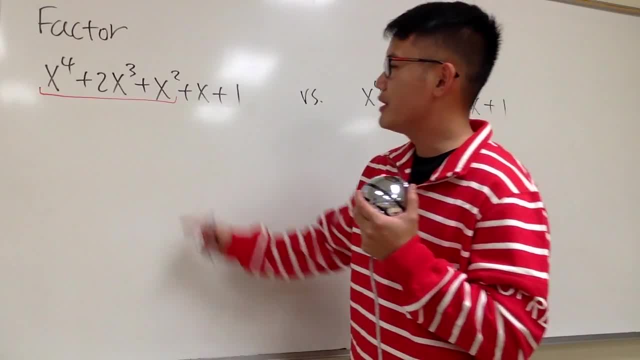 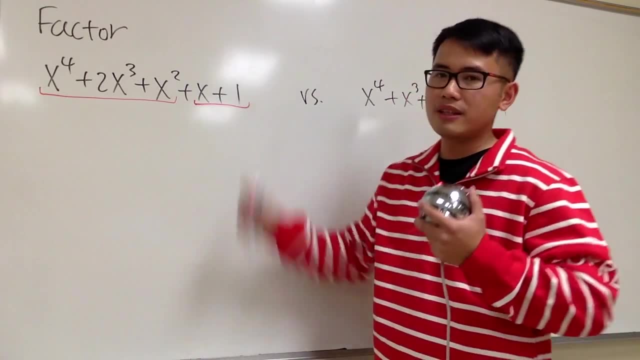 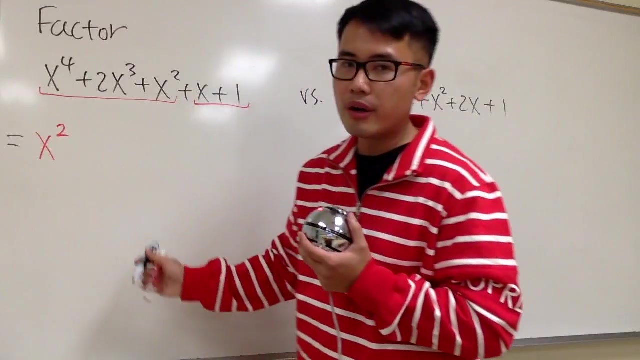 terms like this. Well, why? Because, first of all, I can factor out x squared right. That's good, and without being done, let's group the last two like this then, and let's see what do we get. For these three terms, we can factor out x to the second power. 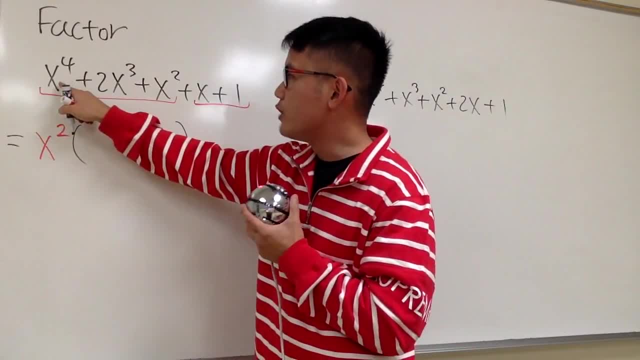 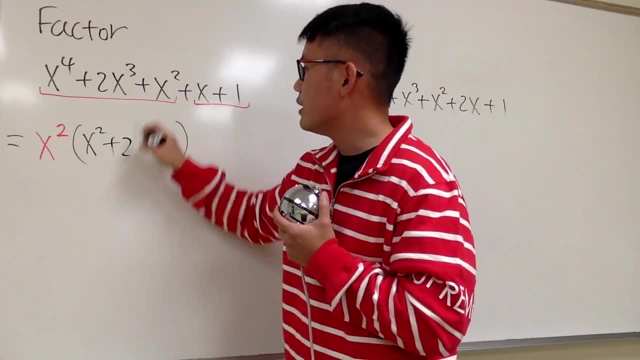 and then for the left over. well, for the first term, originally it was x to the fourth, but we took the two out right. So we have x squared, and then we add the two. we have x to the third. 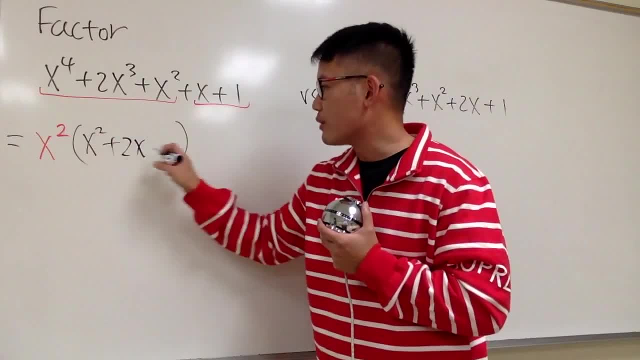 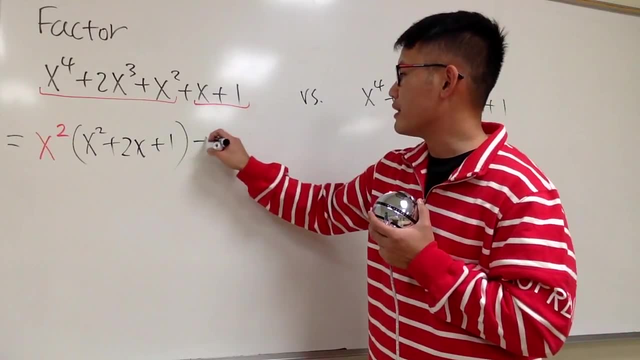 we can factor out two of them, so x to the first. the x squared was out, so plus one, just like this, right? So that's the progress. and then let me write down: plus x, plus one. What can we factor? 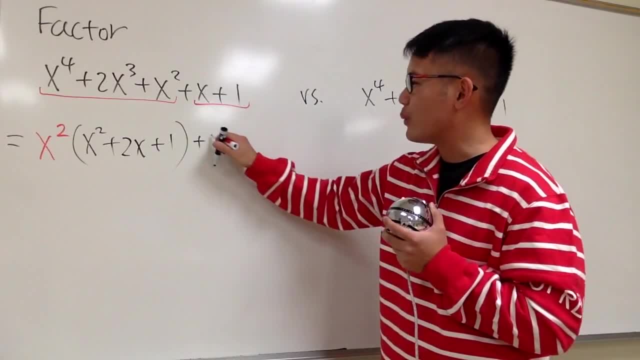 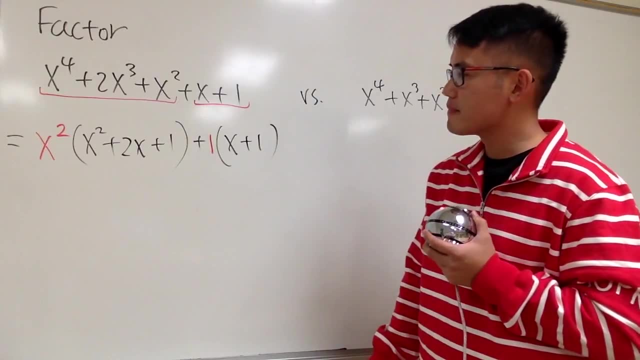 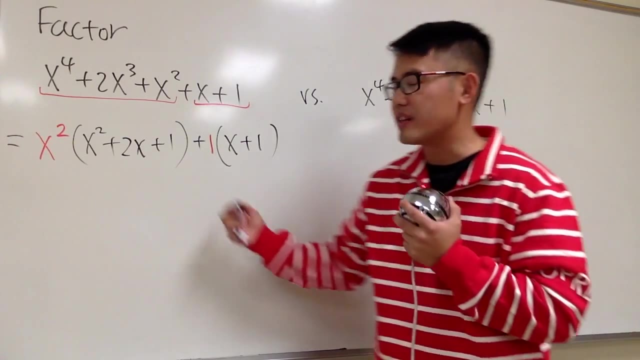 out Nothing too much, right? So let me just factor out a one, and then let me put parentheses around this x plus one, like that. Well, this entire parentheses in black and this entire black. they are not the same, so we cannot factor things out yet, right? however, as i told you guys, 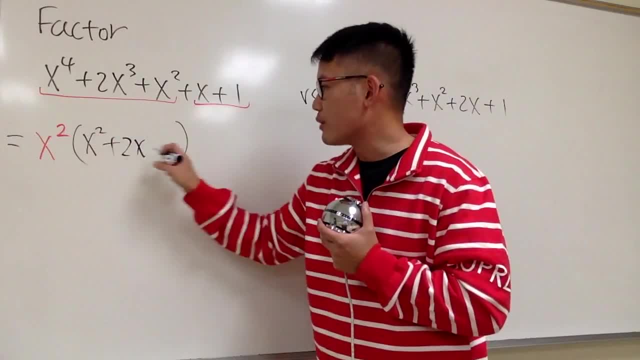 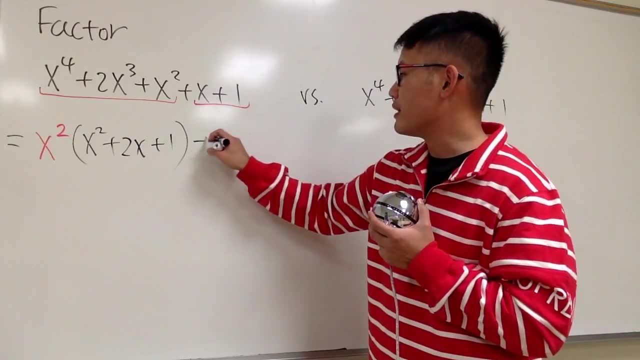 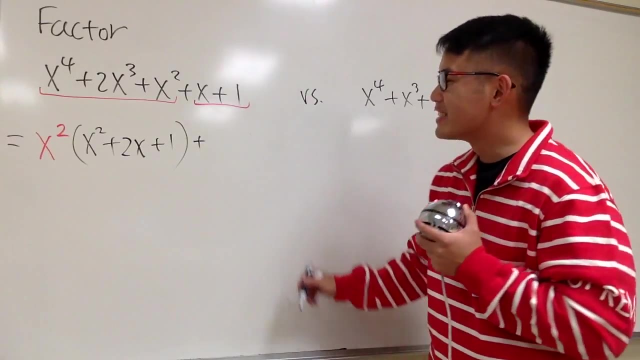 and then we fit out two of them. so x to the first. The x squared was out. so plus one, just like this, right? So that's progress. and then let me write down: plus… X plus one. What can we factor out? Nothing too much, right? So let me just factor out a one. 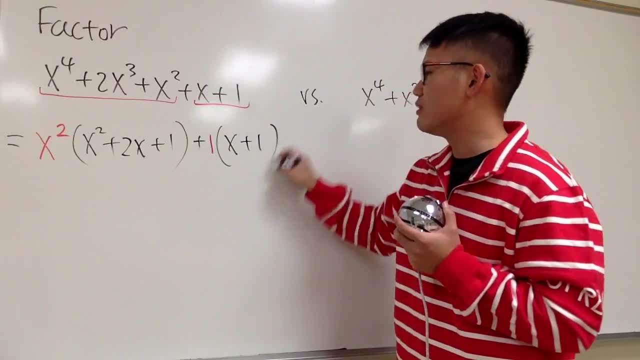 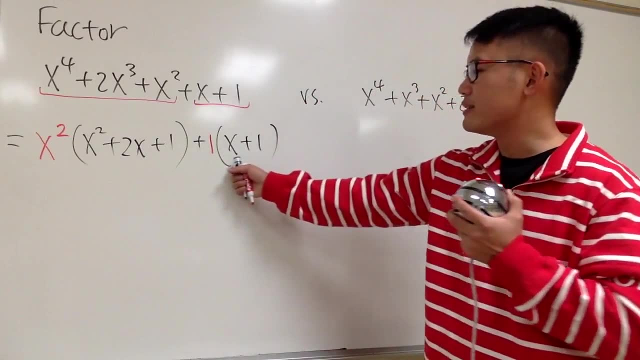 and then let me puteon parentheses around this x plus one like that. Well, this entire parentheses is in black and this entire parentheses is in black and this entire parentheses black. they are not the same, so we cannot factor things out yet, right? however, as i told you guys, 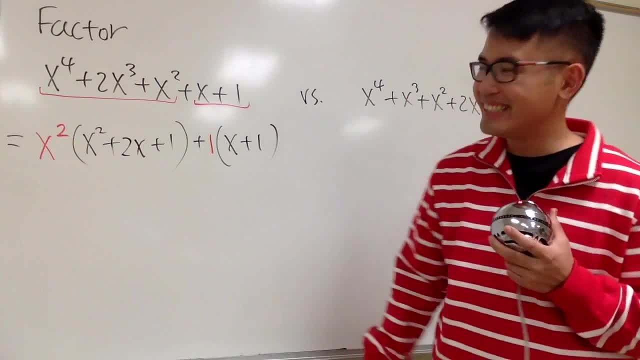 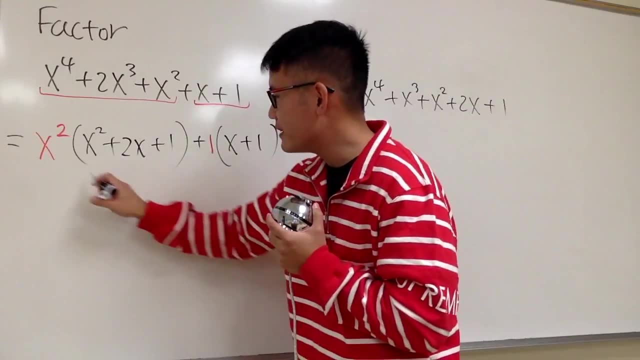 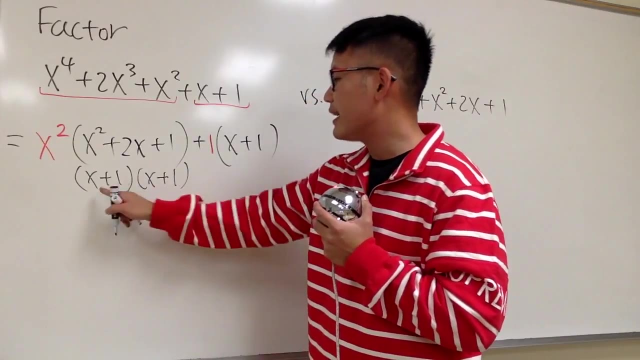 earlier. these questions are well designed it. look at this right here: x squared plus 2x plus 1. what can we do with it? well, we can factor this and this is going to give us x plus 1 times x plus 1. i know this is the same as x plus 1 square, but it would be better for me to write them down. 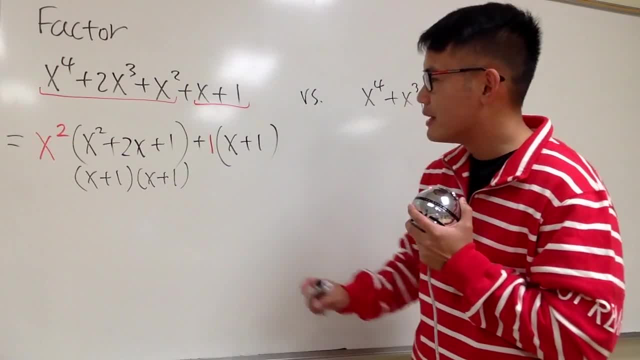 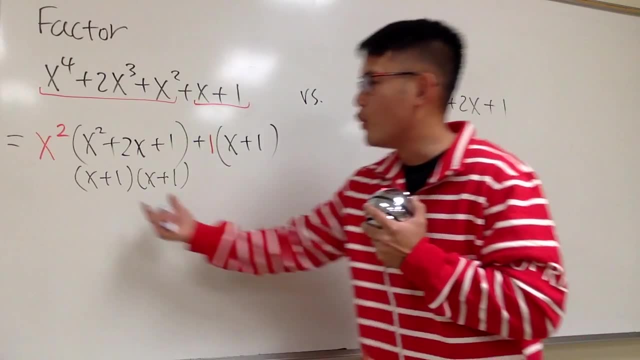 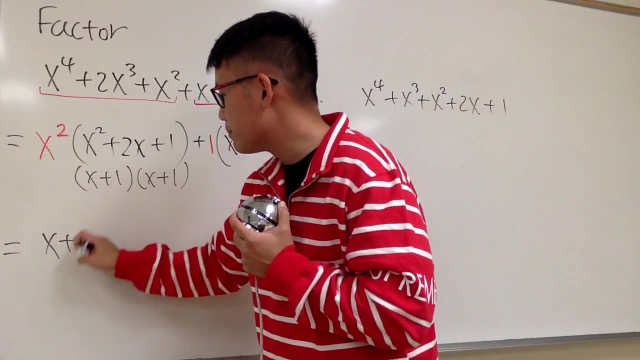 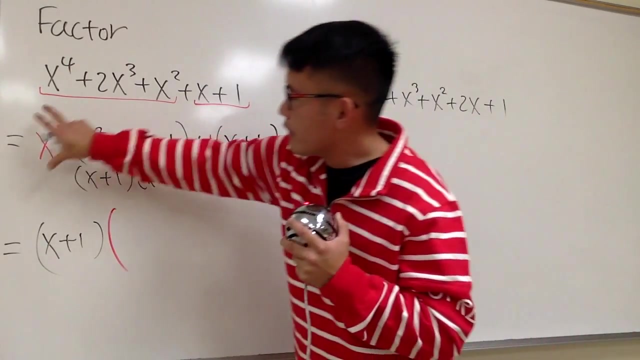 separately, like this for now, and we see that i have an x plus 1 right here and this is also an x plus 1. that means i can factor out one of this, factor out right. so we will do that. let me factor out x plus 1 and then let me put down the left over in this big parentheses for the first part. 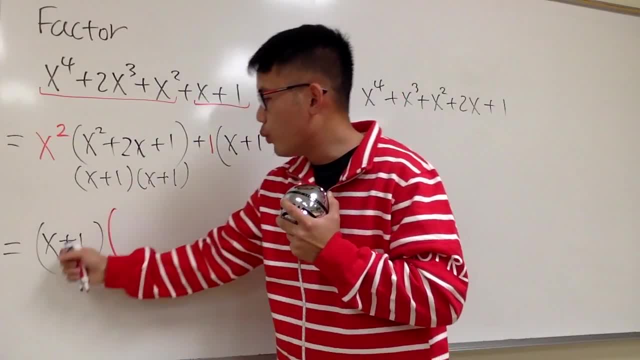 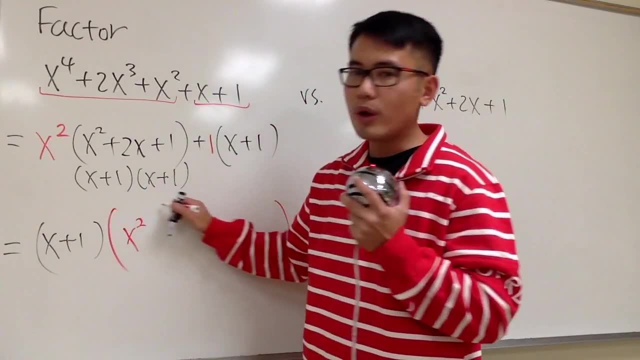 here. okay, before this addition sign, we took one of the x plus 1 out. that means we have the x squared right here still left, and then we have another one right here. so let me put that down. this right here is the one that we still have left: x plus 1. i'll put. 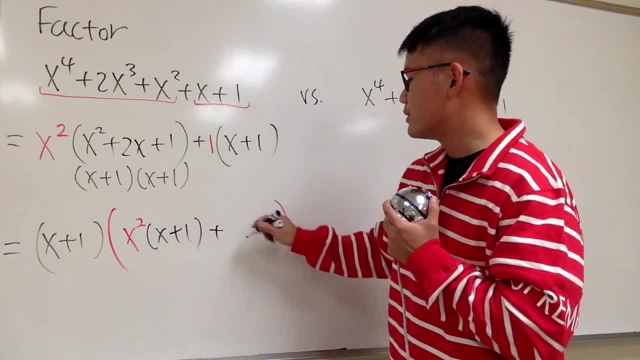 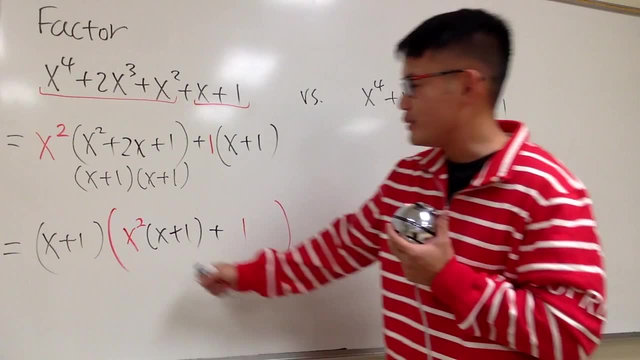 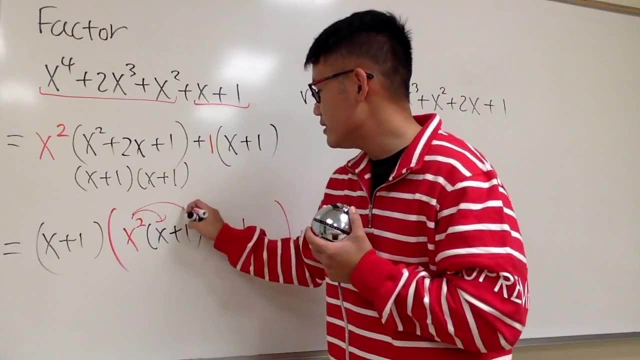 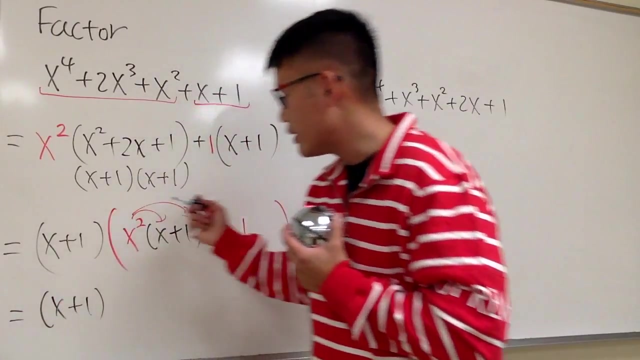 on black, and then we add this one, right, and you see we have a factor times another thing, we factored it. but then the usual deal is that at the inside here- let me just try to combine terms, let me just distribute this into the parentheses: x, squared times that, and actually we're done. we have an x plus 1, all the. 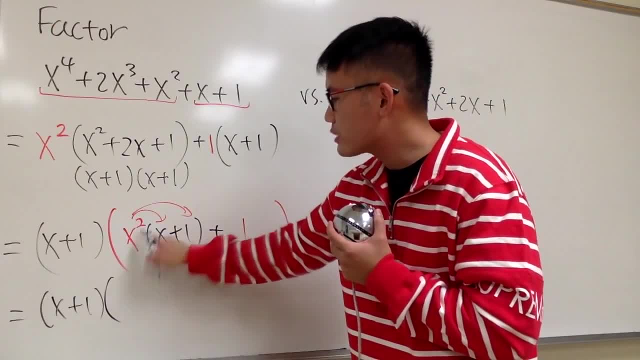 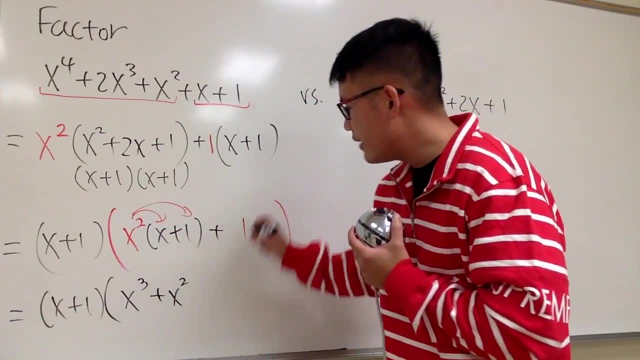 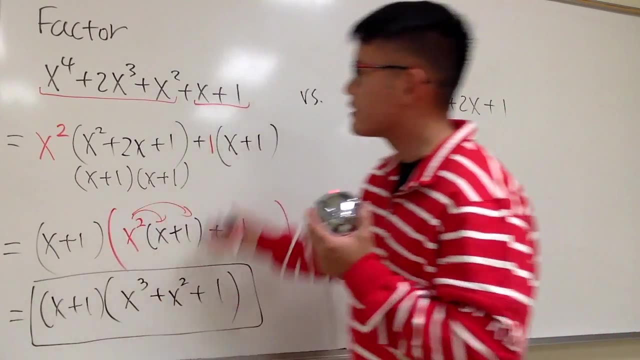 way in the front, and then the big parentheses. it's going to give us x squared times x. that's x to the third power. x squared times 1 is plus x squared, and then we have a plus 1- parentheses times parentheses. look at that. this is how we can factor a finite polynomial right. 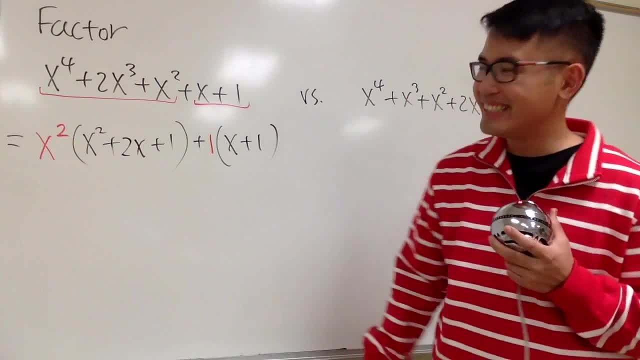 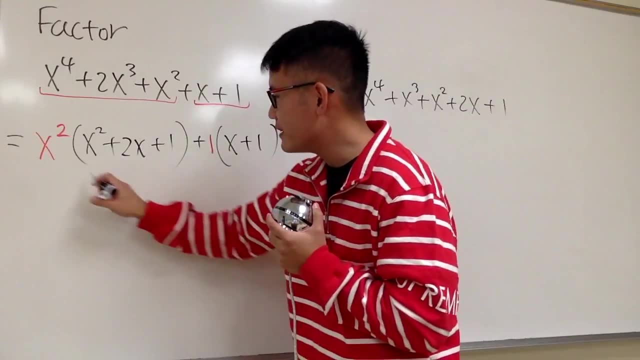 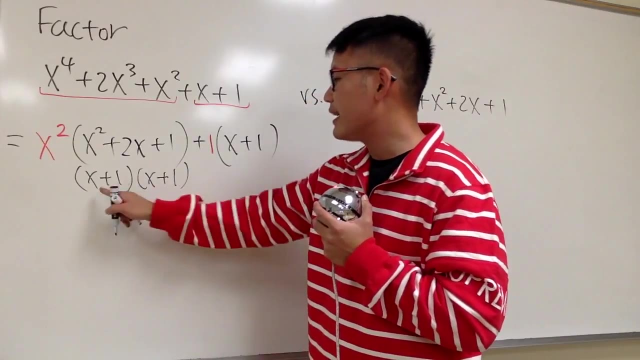 earlier. these questions are well designed it. look at this right here: x squared plus 2x plus 1. what can we do with it? well, we can factor this and this is going to give us x plus 1 times x plus 1. i know this is the same as x plus 1 square, but it would be better for me to write them down. 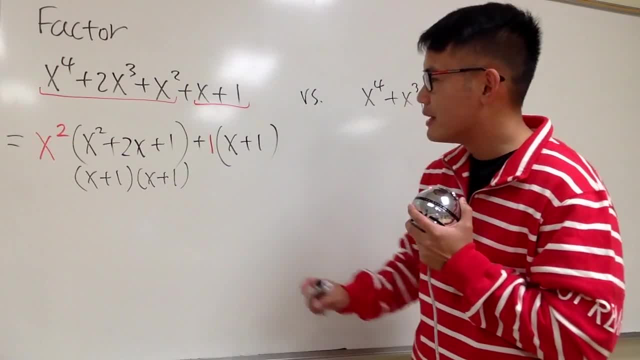 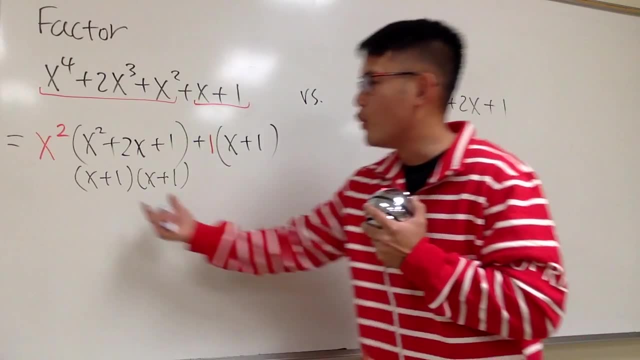 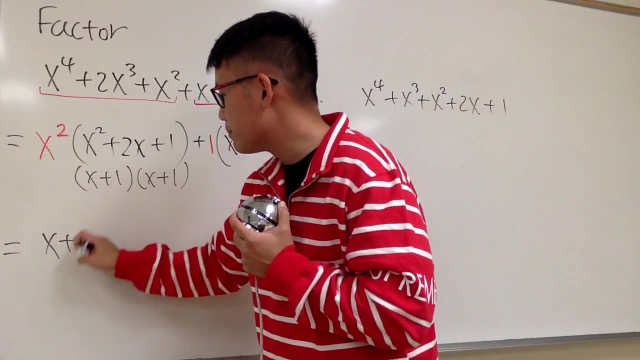 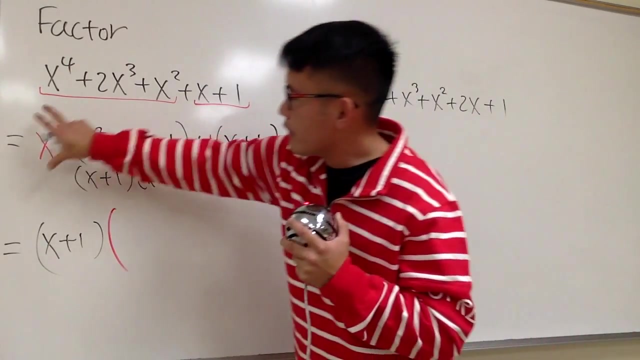 separately, like this for now, and we see that i have an x plus 1 right here and this is also an x plus 1. that means i can factor out one of this, factor out right. so we will do that. let me factor out x plus 1 and then let me put down the left over in this big parentheses for the first part. 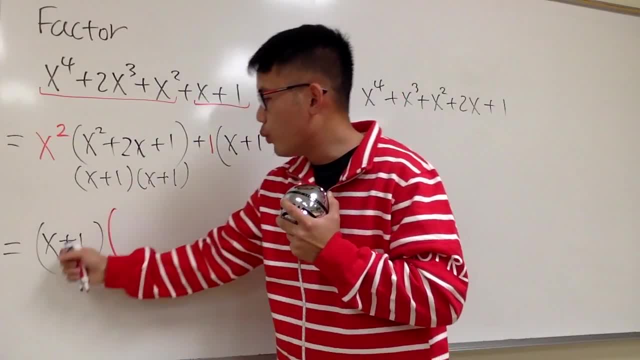 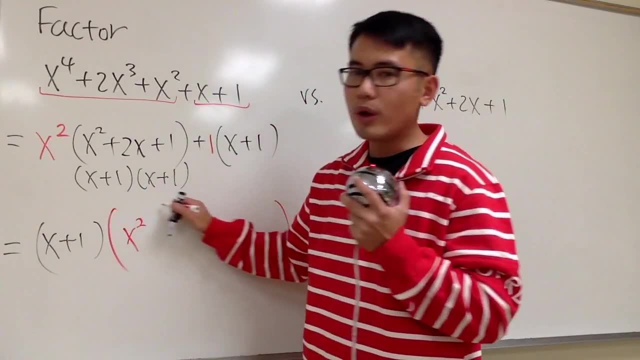 here. okay, before this addition sign, we took one of the x plus 1 out. that means we have the x squared right here still left, and then we have another one right here. so let me put that down. this right here is the one that we still have left: x plus 1. i'll put. 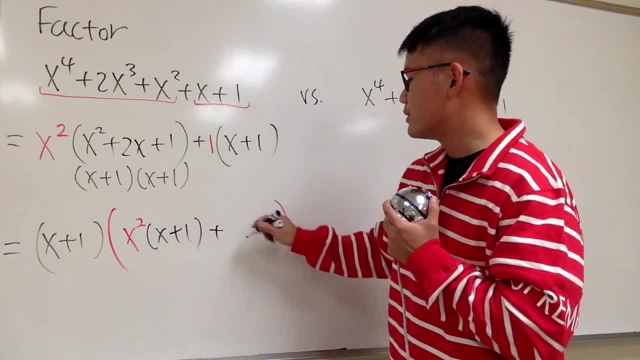 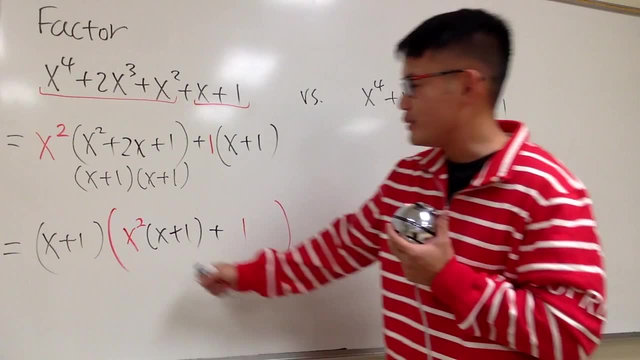 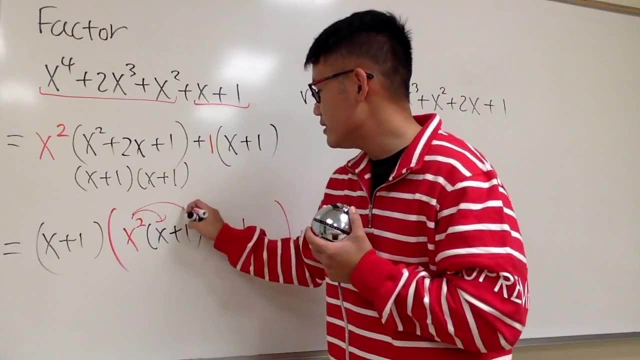 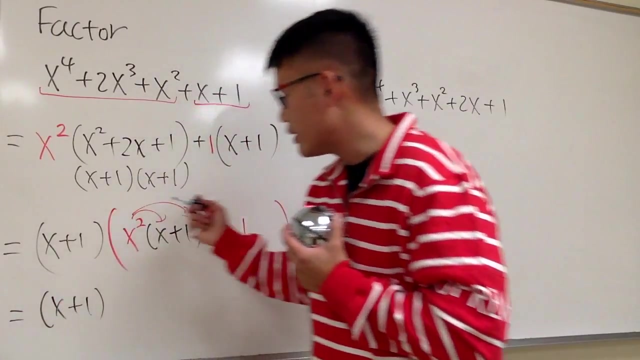 on black, and then we add this one, right, and you see we have a factor times another thing, we factored it. but then the usual deal is that at the inside here- let me just try to combine terms, let me just distribute this into the parentheses: x, squared times that, and actually we're done. we have an x plus 1, all the. 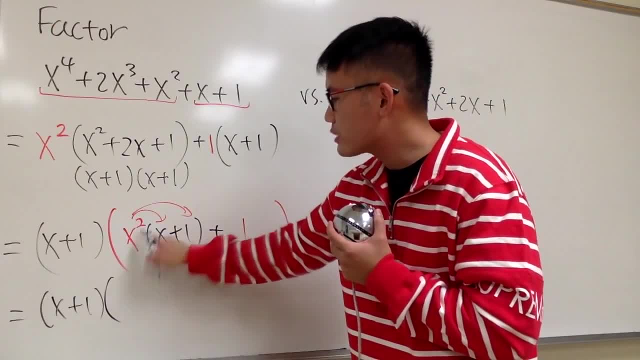 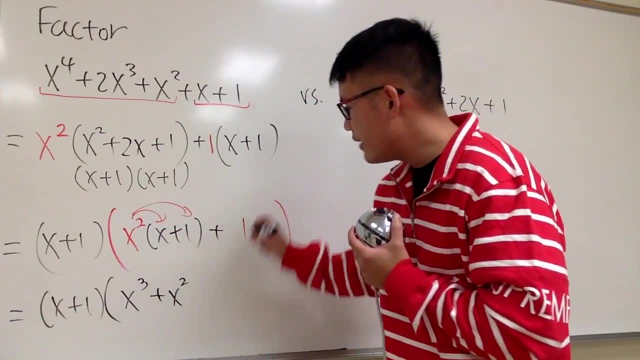 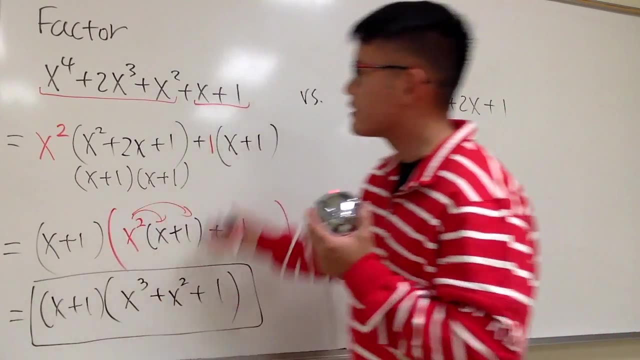 way in the front, and then the big parentheses. it's going to give us x squared times x. that's x to the third power. x squared times 1 is plus x squared, and then we have a plus 1- parentheses times parentheses. look at that. this is how we can factor a finite polynomial right. 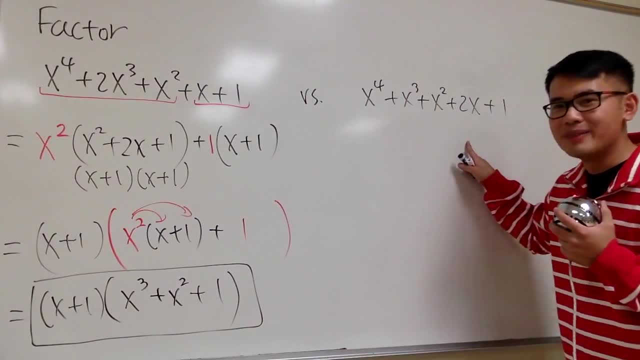 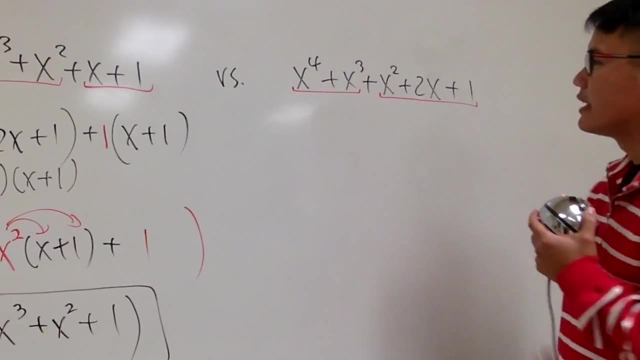 how would you do the second one? i am going to prove the first two like this and then go to the second thing like that, and you'll see for this two, right here, i can back up x to the third power and then we can get: this is x plus. 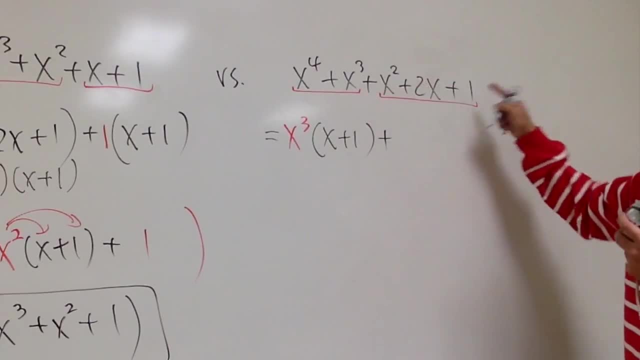 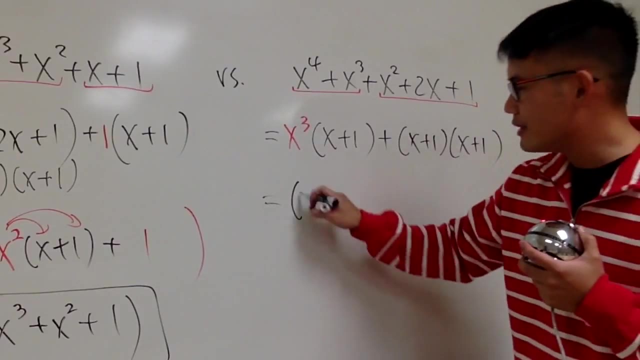 one right. and then i'm going to bring the sign in the middle: x squared plus two. x plus one. what can we do with that? well, we can factor it x plus one times another, x plus one. and look at this: we have x plus one here. x plus one here. we can factor the out: x plus one left over piece. here we have x to.